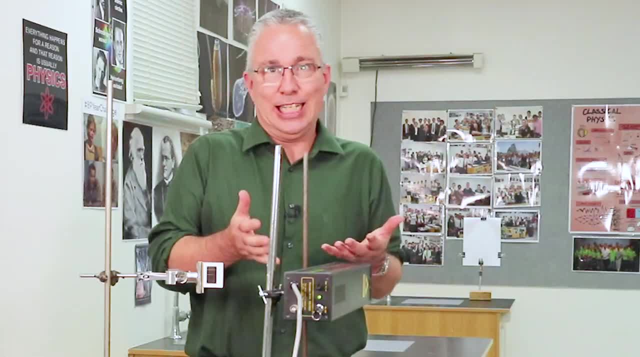 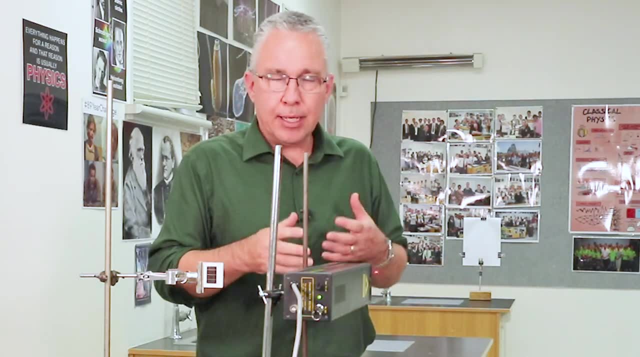 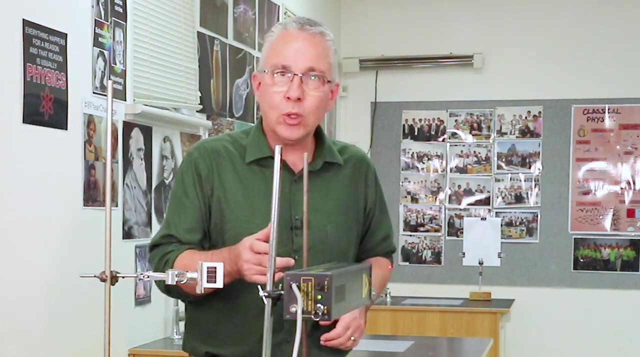 So here I have a helium neon laser. Now, this is clearly a bit bigger than your standard tiny pen-type laser, and this has been around for quite some time, but it provides us a really good, strong laser beam And in this case it's producing red, monochromatic light, and if you look into the distance, you will see a white card. 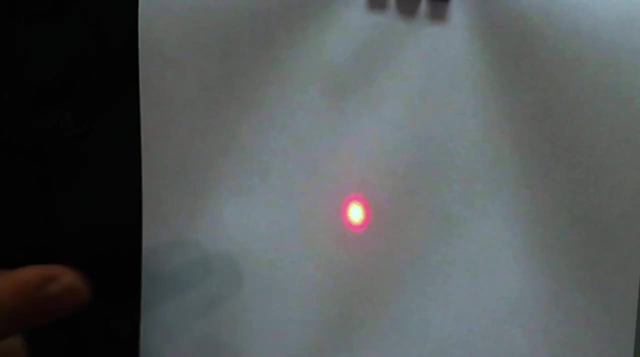 and that white card has got the laser spot on it. So here is our bright spot. It looks grainy to you. That's not because there's something grainy about the light. That's simply because the light is interacting with the surface of the paper. 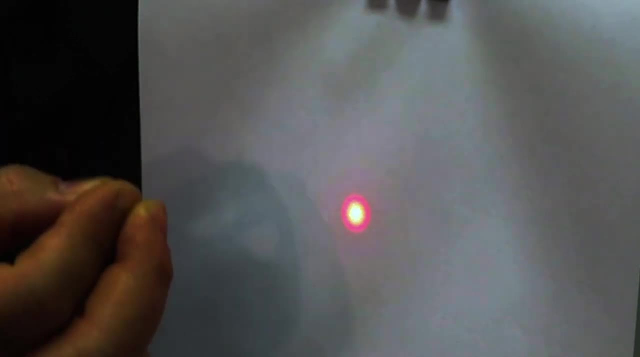 and because the paper is uneven, you're getting reflections from the paper that are coming to you now- not completely all in phase- and as a result, you're going to get this grainy feature here into the bright spot. So now let's have a look when we place in front of it. 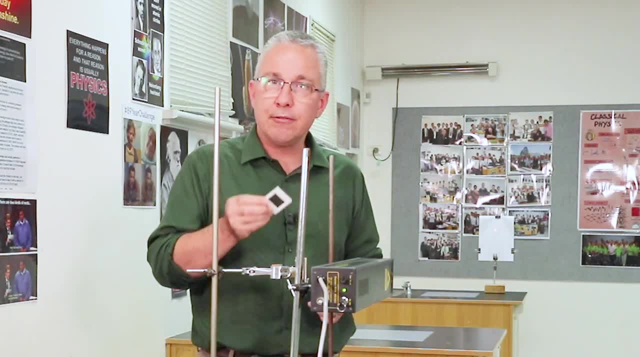 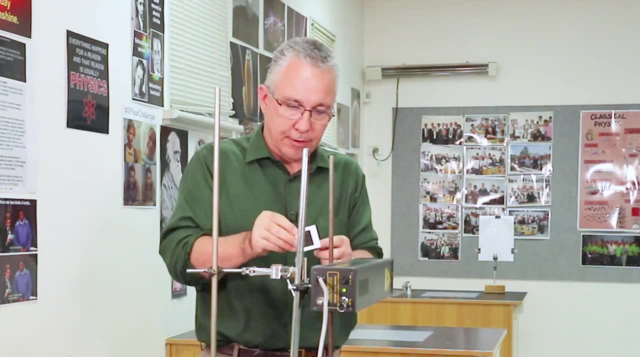 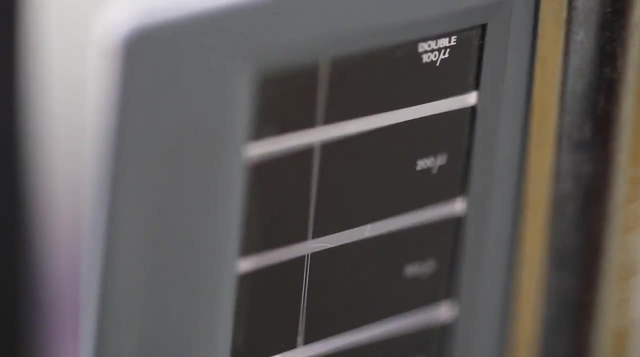 This is the Now. what I have in front of me here is a slide that has four versions of some slits embedded, and it's a vertical line. So what I have here is at the top, I have two slits that are separated by 100 microns or 100 micrometers. Then I have one 200 microns, 300 microns, and then I have a single slit that is a single particular distance and we're not going to use that one. We're going to use a slit that is a single particular distance and we're not going to use that one. 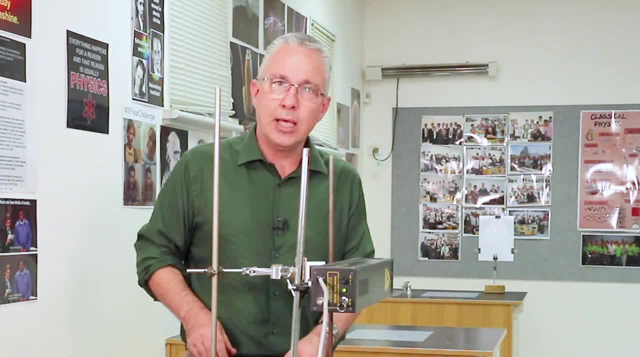 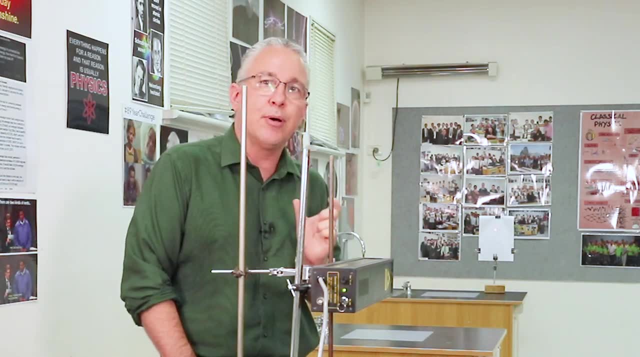 the one that is separated by 300 micrometers, and I'm going to place that in front of my laser, and what happens, of course, is that the light hits both slits, and so, in effect, we're generating two separate sources, and both of those of 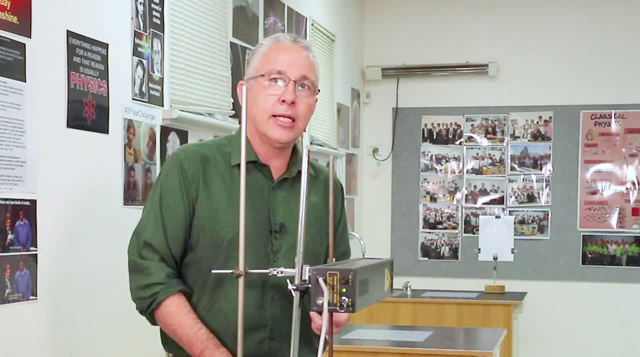 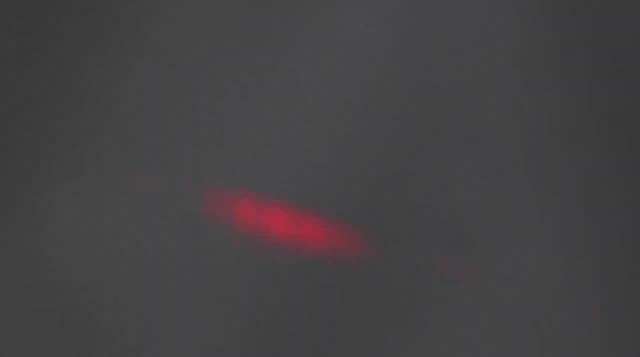 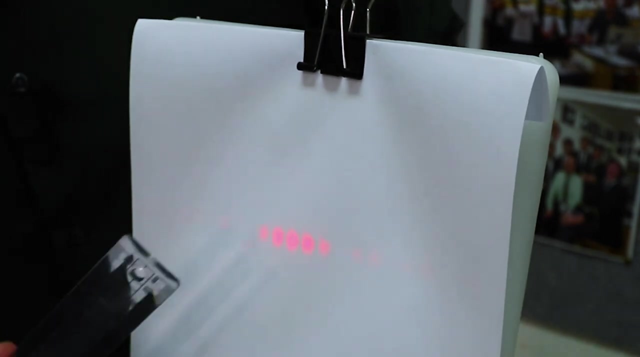 course, are going to be coherent, that is, they're going to be in phase and they're going to be obviously the same frequency and same wavelength of light. so what you can see are a series of bright and dark areas, and this one here is the position of my original dot. and then, on either side, you see a dark. 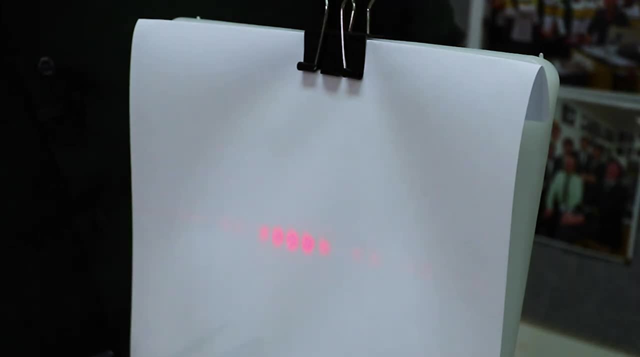 region and then again bright regions, and what's happening is, as we're getting, constructive interference at each of the bright spots and destructive interference at the dark spots. in other words, light is reaching from either slit on both of those dark spots there, but because they are out of phase, they are cancelling out, and so we're. 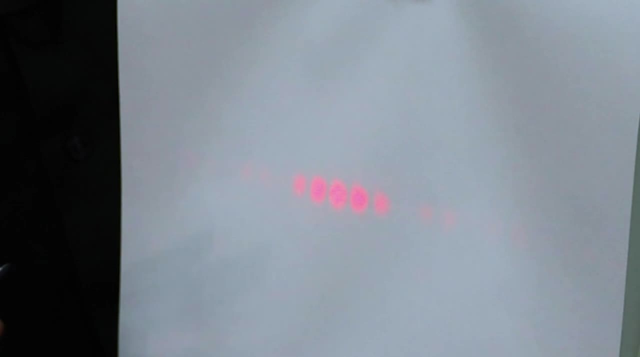 getting these dark spots. So what we're going to do now is we're going to measure the distance between the first bright spot, which is the central one, and the second spot, which is really what we call our first order. So it's our first spot after the central spot, and I've got here a small ruler and we're going to 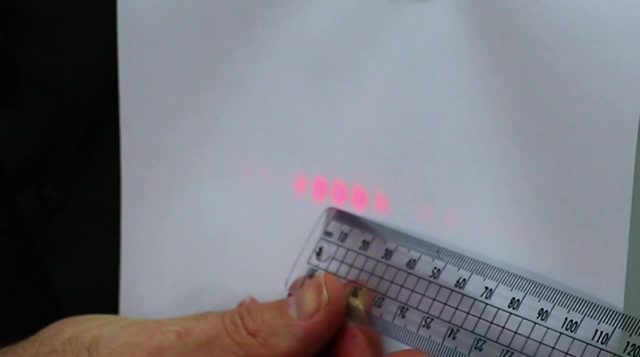 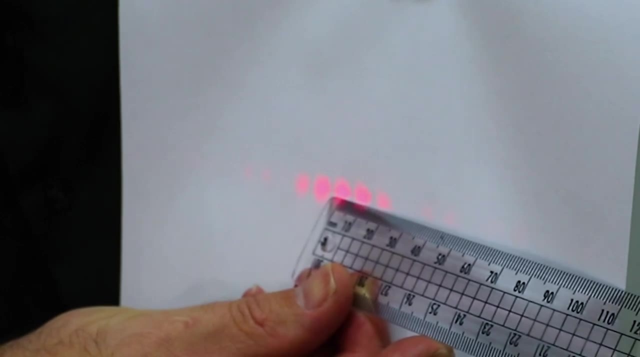 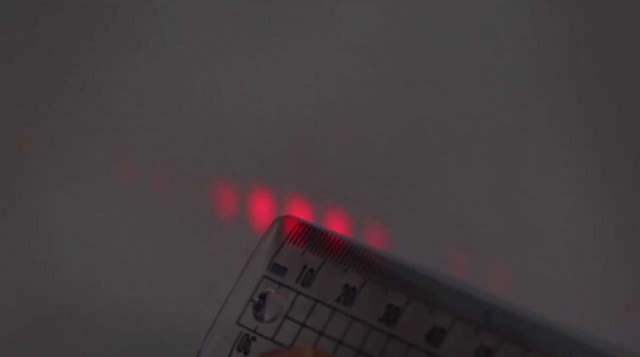 try, to our best of ability, measure the width or the distance between the two spots and if I try to place it directly in center, you can see I'm going to get. in this case, I would estimate. the best estimate I have is 0.8 of a centimeter. 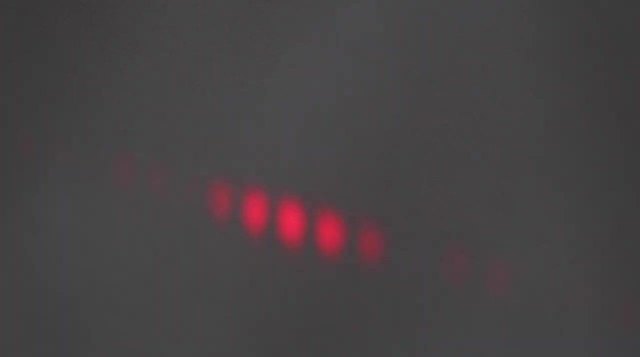 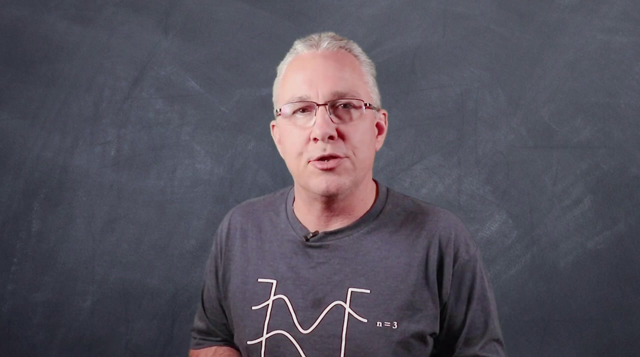 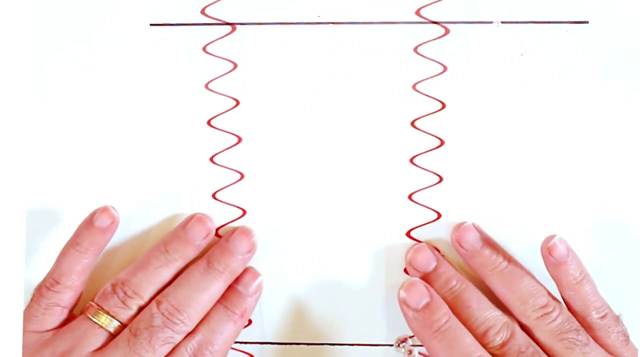 or 8 millimeters, and we're going to use that in our calculation. So before we start looking at the mathematics of double slit interference, let me provide you with a simple demonstration to show why we get regions of constructive and destructive interference. So what I have here is a very simple demonstration to help you. 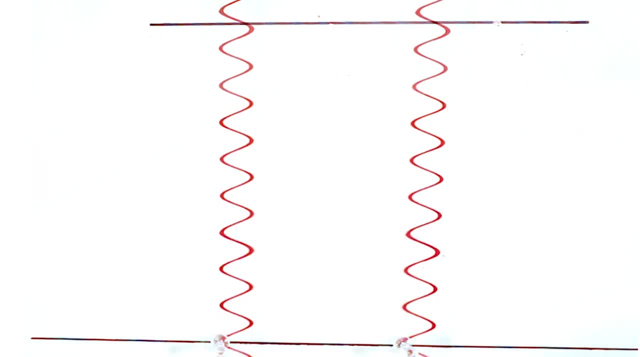 understand how interference works, and I have these two rays coming out from these two pins. Now, the pins represents our slits, and you'll notice my two rays are completely in phase and we've, of course, got the same wavelength. so, as a result, you could argue that these two rays are coherent, they're in phase and of. 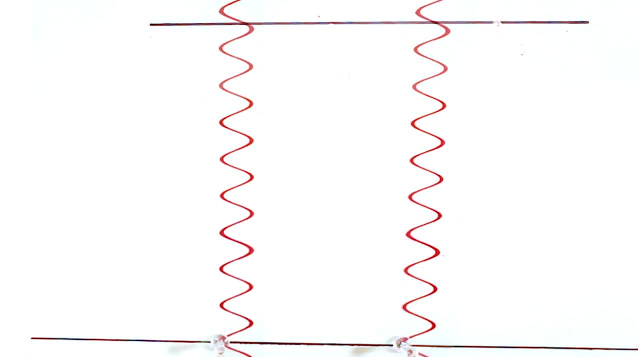 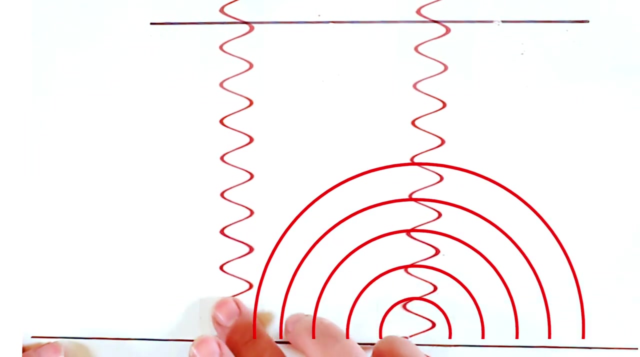 course, the same wavelength and frequency, And the line represents our screen. Now, in reality, of course, if light is coming out from this slit, then it's all of these rays occurring and that will produce these wave fronts that are concentric circles, and that's true for this here as well. 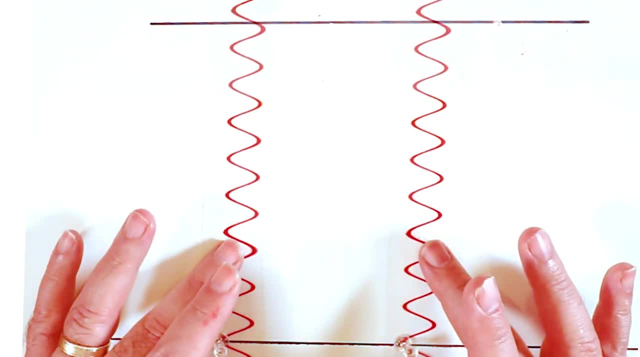 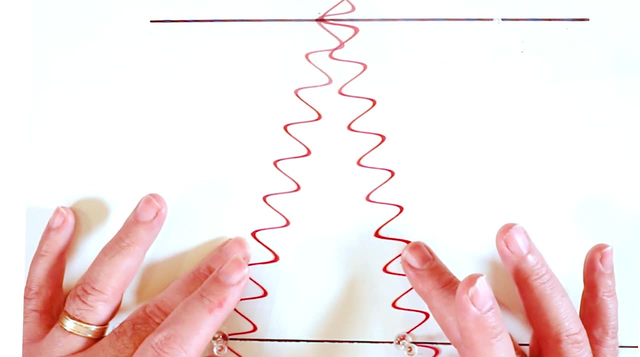 But we're only going to examine two of them so that we can see what happens when they actually interact or interfere with each other. Now there is a point right in the middle, and that's this point right there, where you'll notice that we have complete overlapping. 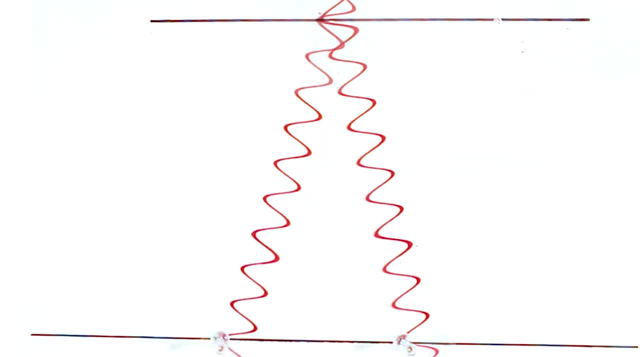 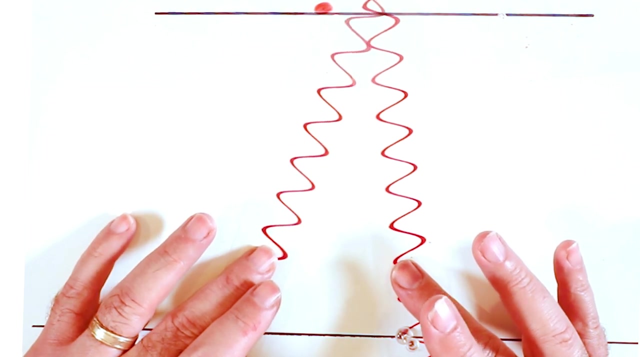 And they're completely in phase here, and that means this wave and this wave add up, we get constructive interference, and so we're going to get a nice bright spot right there. Now, if I, however, move this one in that direction as well as that in that direction, you'll notice the common point, and that's roughly in this. 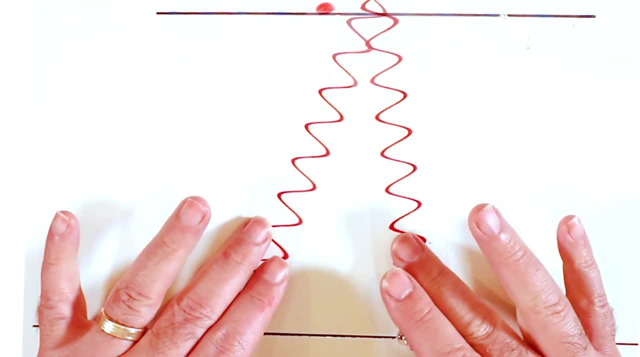 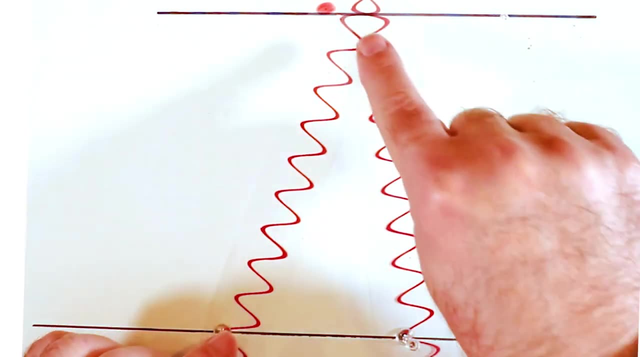 position over here where I've got, let's say, the downhill section of one and the uphill section of the other. they're cancelling out. so that's out of phase right there. So we get a dark spot there, but if we move along we'll find there'll be. 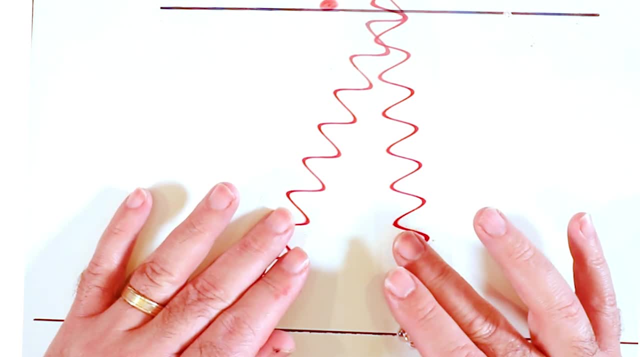 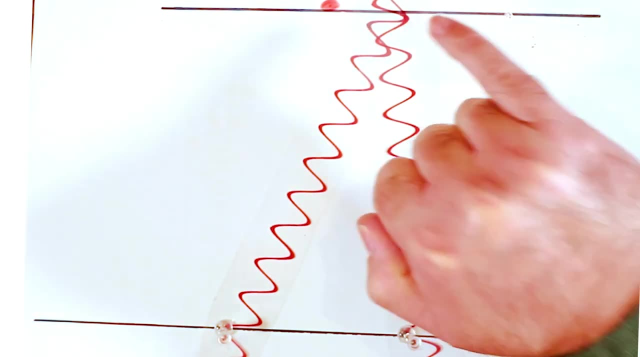 another spot, and it's roughly in this position here where- and because of my little setup here that's not completely aligned, not perfect, but nonetheless, we're getting heat constructive interference. How do I know? Well, I've got one, two, three, four, five, six, seven, eight, nine and a half wavelengths here. 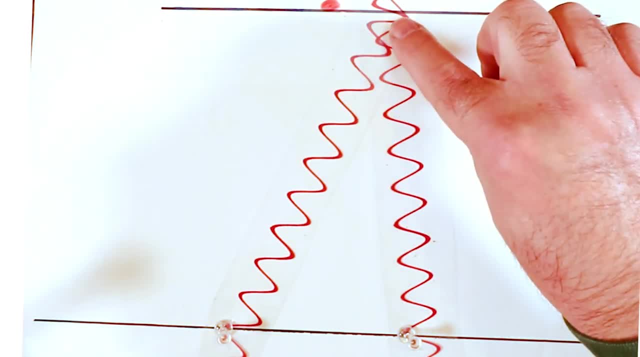 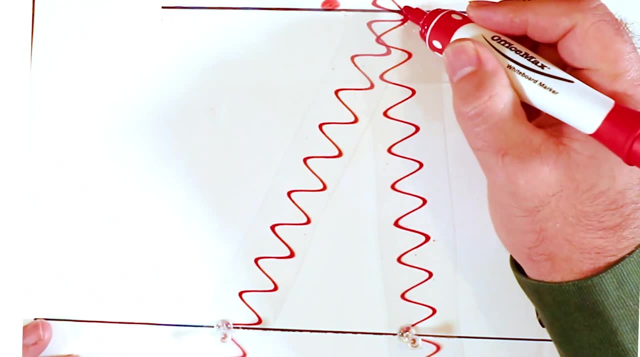 and I've got one, two, three, four, five, six, seven, eight and a half wavelengths here. So you've got now a path difference of one full wavelength And so that there becomes a bright spot because we're getting constructive. 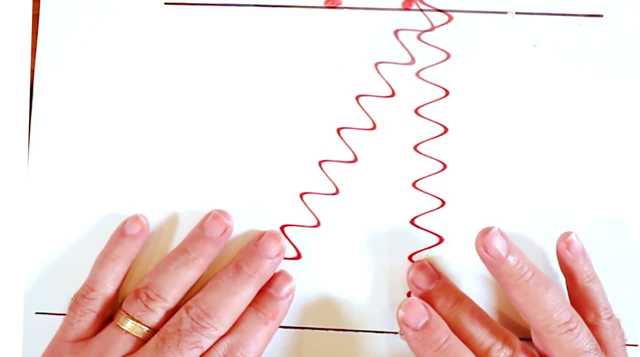 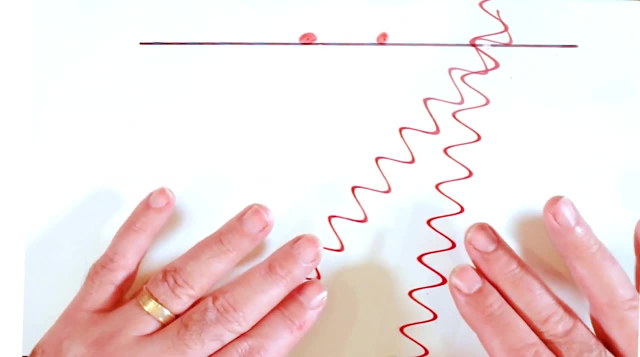 interference at that point. If we keep going that process along, you'll see that eventually I'm going to get a point where I'm going to get at another one and I'm going to get one that's sitting. let's say here, Let's have a look at the. 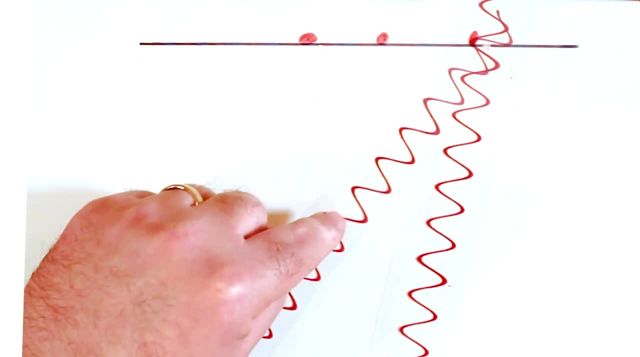 path differences. I've got one, two, three, four, five, six, seven, eight, nine, ten eleven from this side and one, two, three, four, five, six, seven, eight, nine, and so this case is clearly a. 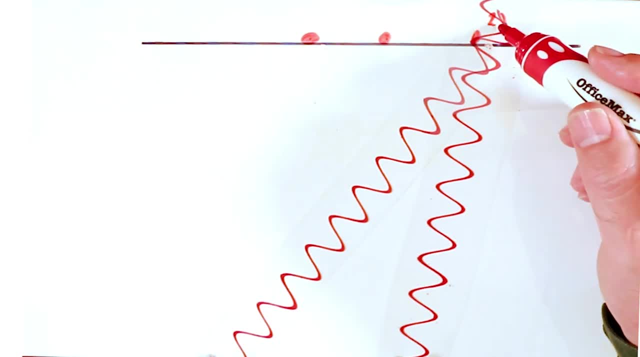 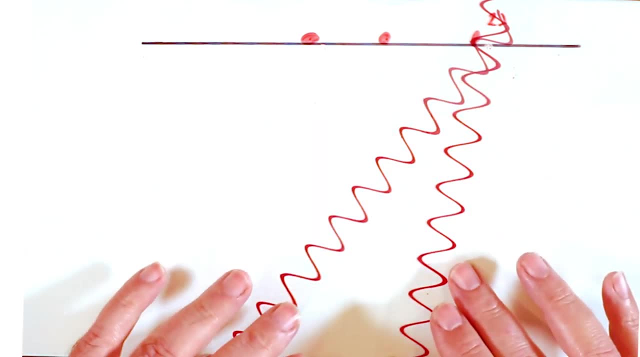 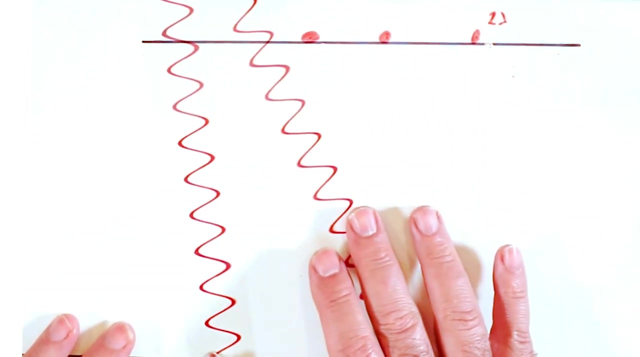 path difference of two wavelengths, but they're in phase, We're getting constructive interference and so therefore we have a bright spot over here and of course, that's going to be mirrored on this side as well. and, again, as we said, it's because the waves are arriving in phase and where they're, 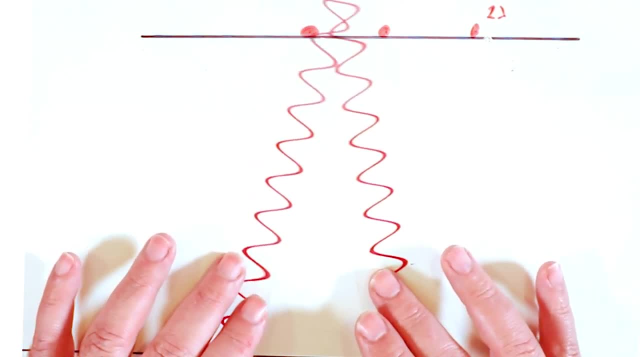 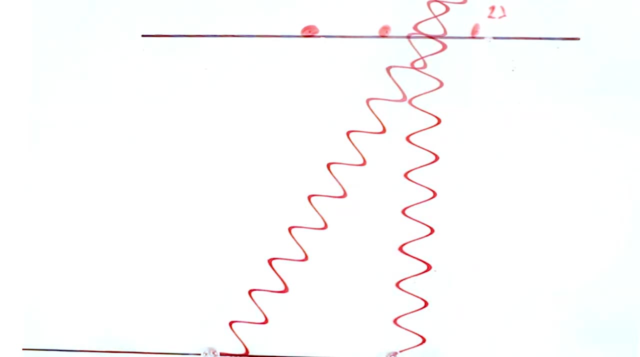 arriving out of phase, as in a difference of half a wavelength. so say, in here we've got a difference of about half a wavelength, right there we're going to get destructive interference here, and so we do not get any bright spot right like so, and so that should help you. now let's move these. 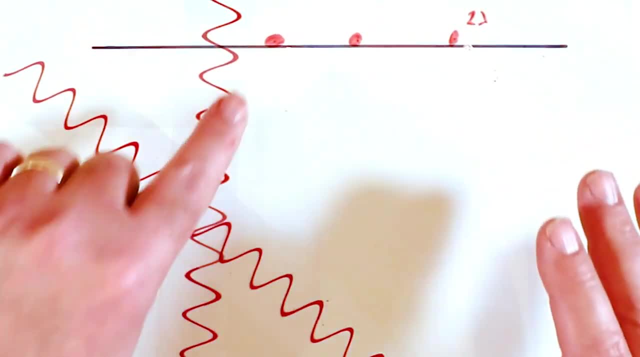 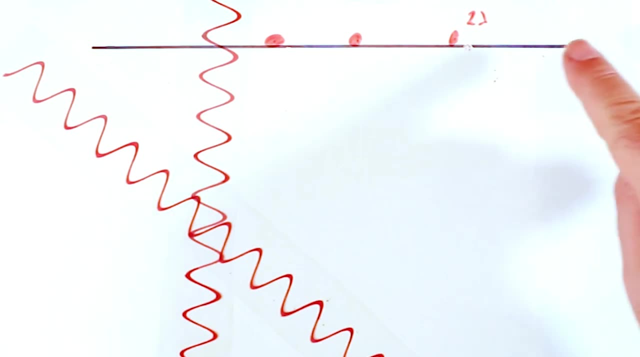 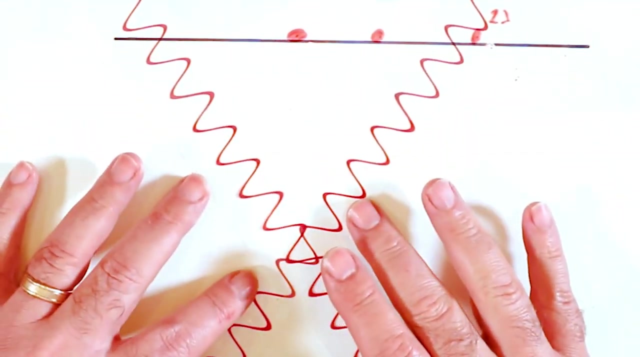 down the road why we get these bright spots, one in the dead center and then, of course, successive ones as we go on. So one wavelength difference, two wavelength difference, and well, of course, we'll get three wavelength difference, but because this one here is now travelling significantly further than this one. 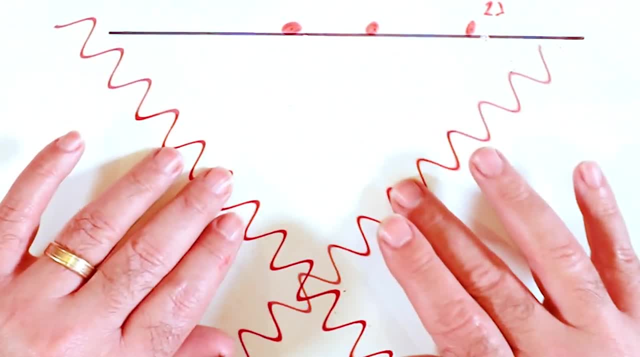 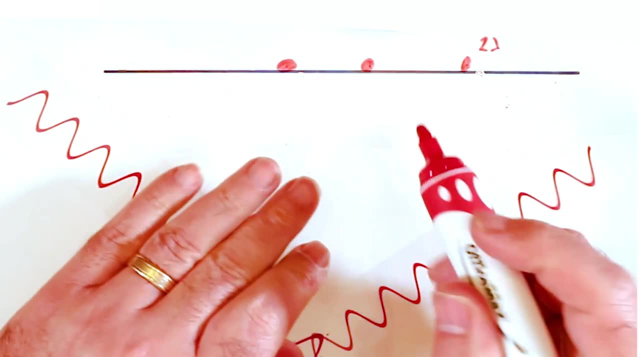 over here. what we will find- this right here is Now we're now- is that the intensity of these particular spots will decrease. now it's not gonna be nice and clean. chances are we're going to get a really bright spot over here. it's going to peter off and we're getting a sort of a bright spot. 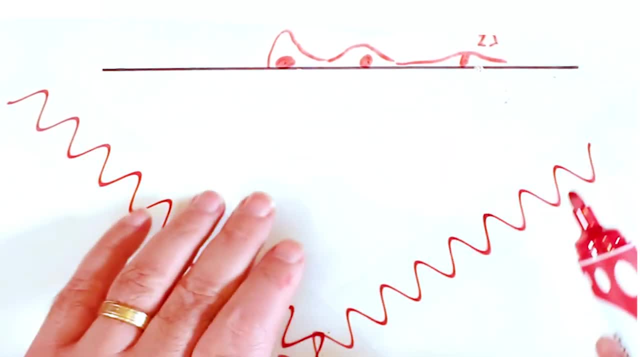 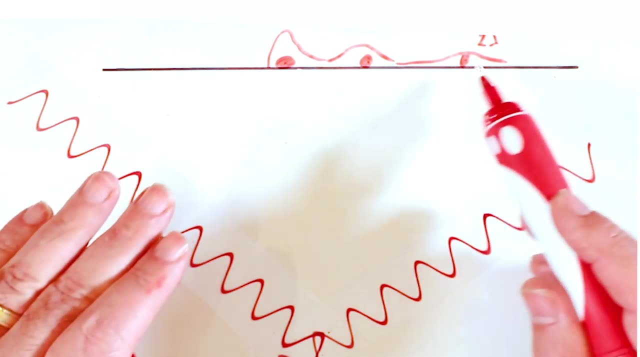 like this, and then it's going to get a sort of bright spot like this, that is, it's going to be obviously a little bit of destructive, constructive interference and it's going to be not a clear spot but a more of a spread blob, so to speak. 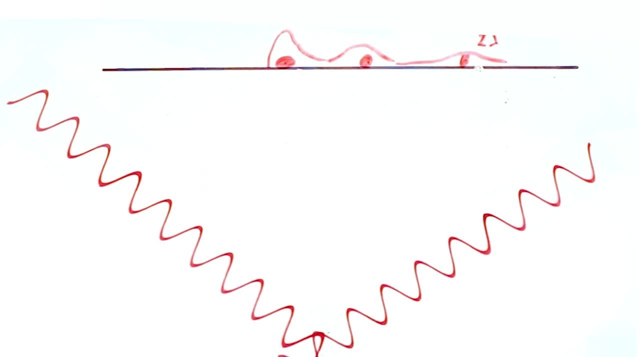 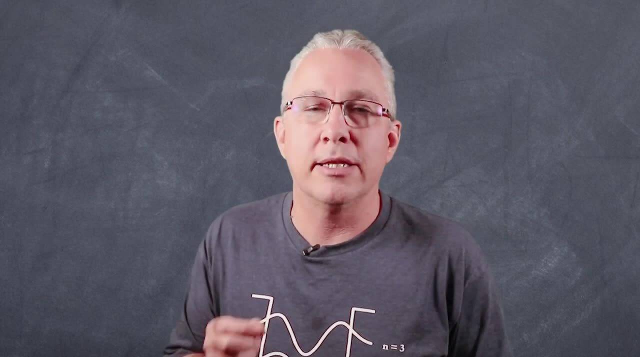 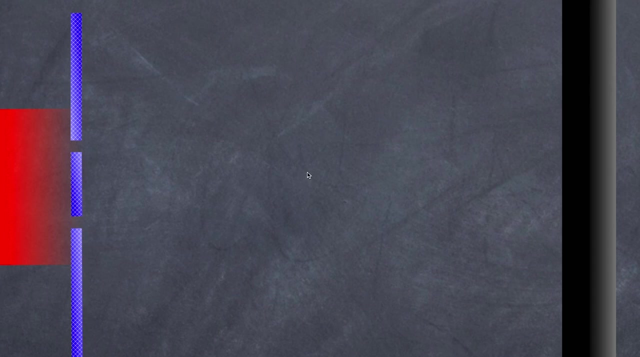 and of course that's mirrored on the other side as well. now that you understand that, let's do a bit of mathematical work and we'll use what we learned to determine the wavelength of my helium neon laser. so one of the hallmarks of Thomas Young's experiment was the definitive evidence to show that. 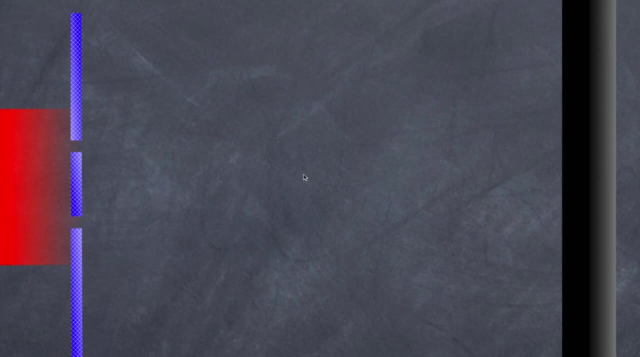 light was a wave and not a particle. now, what would actually happen if light was a particle? well, here I have my light passing through my slits. what would you see on the screen here? well, what you're going to see basically two spots. as the light streams in through particles, it's 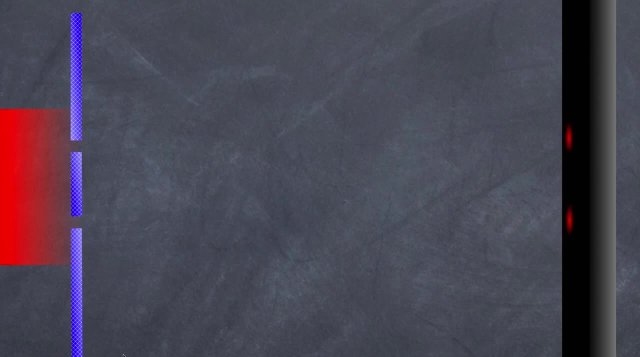 going to give these two bright spots, but we know that's not what happens now. what of course happens, as I've demonstrated already- is is that if you have a wave of light- in this case I have a wavefront of light- we're going to get these two slits. 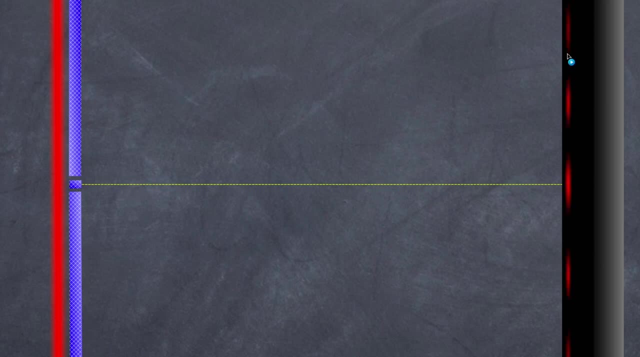 releasing light and what we get is our interference patterns and we have these maxima and, of course, in between these dark areas, you the minima. and what we're going to do now is we're going to examine the mathematics of that so we can establish relationships between the distance. 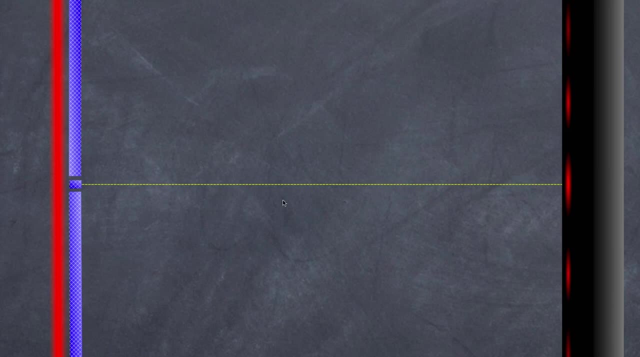 between these maxima, the distance away from the screen, the wavelength of light and also the slit separation. and in order to do that, what we're going to do is we're going to label this a little bit. so, first of all, what we want to do is demonstrate the two paths of light that are coming from both of these slits. 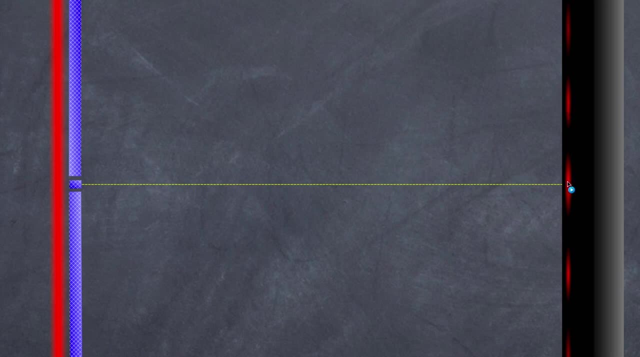 to create this first maxima. we already know that this one here creates an isosceles triangle and really, for us to look at the mathematics, what we want to do is looking at the first maxima. so we have our first path like so, and, of course, 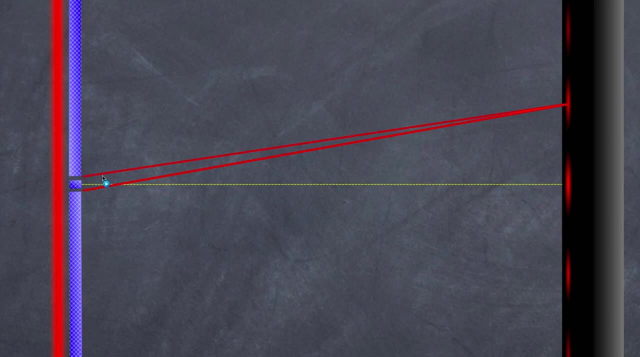 our second path is like this. now, at this point, it's reasonably clear that the top one is slightly shorter than the bottom one, but please understand that these are practically identical. why this is the actually separated, in our case of 300 micrometers, and this distance is measured in multiple meters. 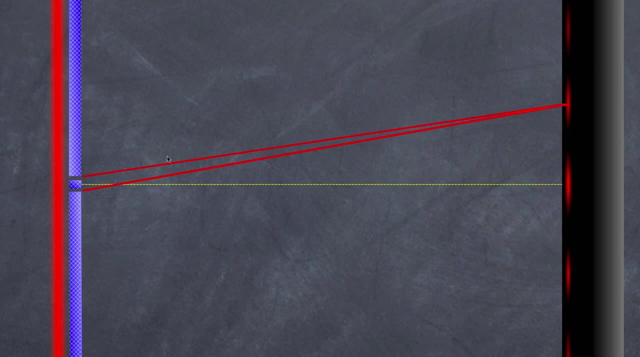 and, as i'll discuss later on, it's over four meters, so these two are really really similar. in fact, what we end up doing is we actually end up drawing a line that is sort of the average between the two, and so we're going to use this yellow one, like so now, this yellow line, we're 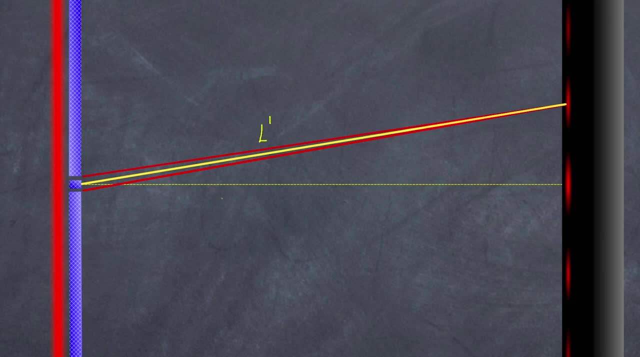 going to give a distance of what we call l- dash, whereas the distance that the dot line is, which is our perpendicular distance to the screen, we're going to call l. and then, finally, we're going to have a distance between these two maxima and we're going to call that y what we're interested in. 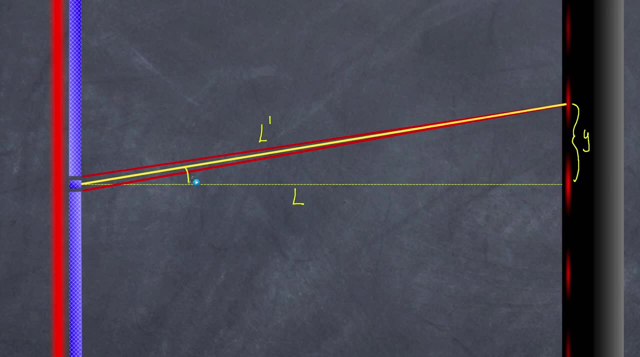 is the angle that we are creating here and this is the angle we're going to discuss at the moment, and you'll see that this angle can be determined because the tan of the angle is going to be simply equal to y over l. that's an important relationship that we're going. 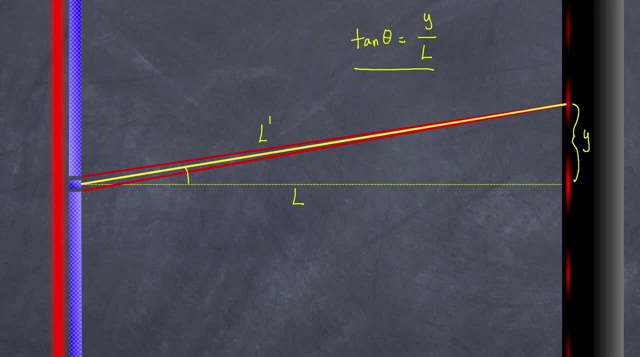 to use for our next particular slide, because what we now want to do is actually look at the path difference and in order to do that we need to sort of have a zoomed in section of just this section here. so now what we do is we look at this close-up section of our light rays. now, these three of 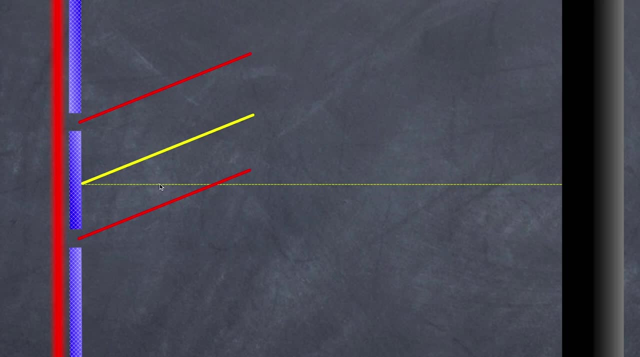 course, are not complete parallel, but for all intents and purposes they are going to be parallel for us. so what we now need to do, we're going to draw a line that is roughly perpendicular to this line. i'm going to draw it like this freehand. now why am i doing that? because this distance here, remember these. 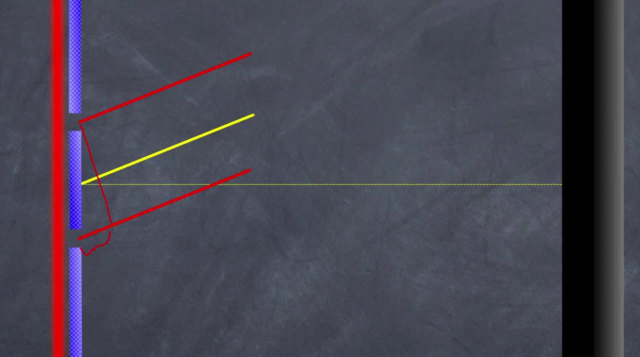 two light rays, the two red light rays, are an example where we get constructive interference. and if you remember from my example, the difference between the top and the bottom is the distance between the top and the bottom, and the distance between the top and the bottom is one complete wavelength. so what we call this is- we often refer to this as the extreme of the- 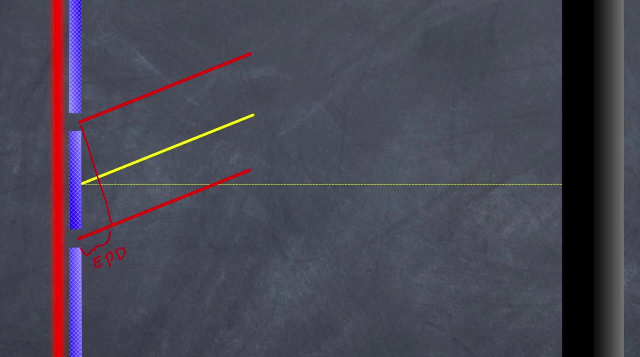 extreme path difference. sometimes it's written like this: but it's equal to one wavelength, because this one is one wavelength shorter, but because they are in phase, we're going to have a difference here of one wavelength. now that means all of a sudden we have a relationship between this wavelength and the slit separation, so our slit separation. 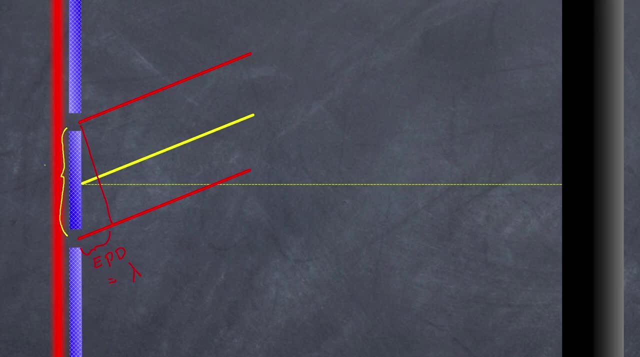 which is this distance. we're going to call this d. the angle here is actually the angle here. it's the same angle. this theta here is this theta here. but now our theta can be determined and you'll see that sine theta is equal to opposite over hypotenuse, which is going to be our wavelength. 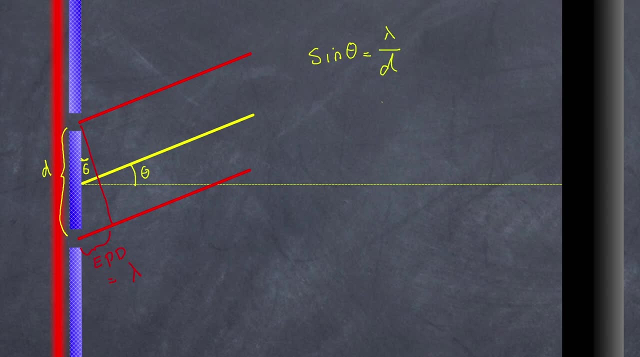 over the distance. so previously we had written that as theta and now we're going to write that as tan. theta is equal to y over l over l, which is, of course our perpendicular distance- notice, i don't even use l dash here- when this angle becomes really small. so in other words, when theta starts to 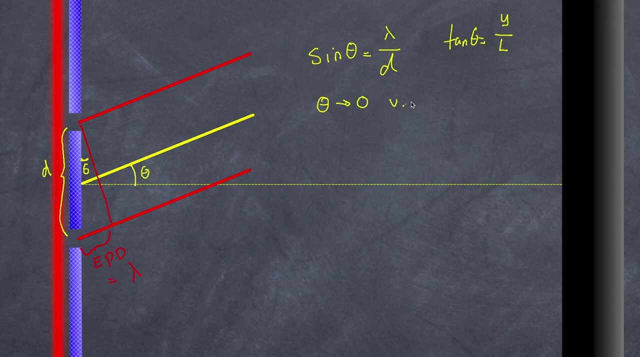 approach zero, or what we say, it's very small. what happens is is that sine theta approximates to tan theta. now, that's significant, because now what we can say is that lambda over d is equal to y over l, and if i clean that up, i get lambda is equal to y, d over l. now, what are those variables? let's remind. 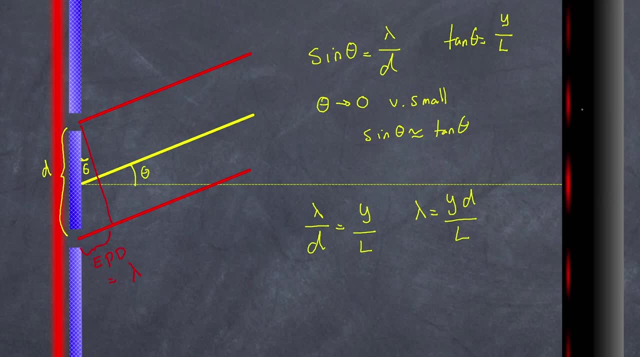 ourselves. our y is that distance here, our y is that distance here, our y is that distance here. our l is the distance from my screen and our d is our slit separation. now, this is only true if this distance is significantly smaller than the path that we have here. 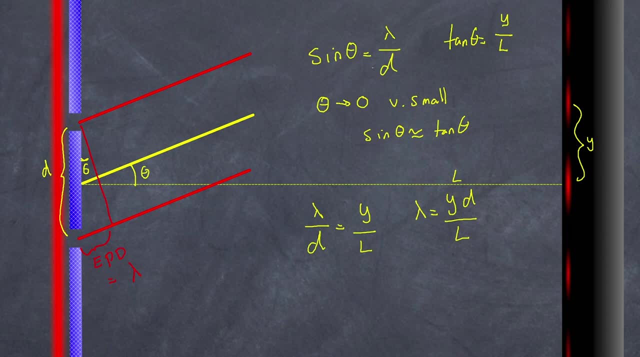 another way to think about this too- and it's often written in the books- is simply looking at this relationship here. and, of course, when we look at that relationship, then lambda is just equal to sine theta. now, of course, that's for the first maximum. so what we often do is that if you have 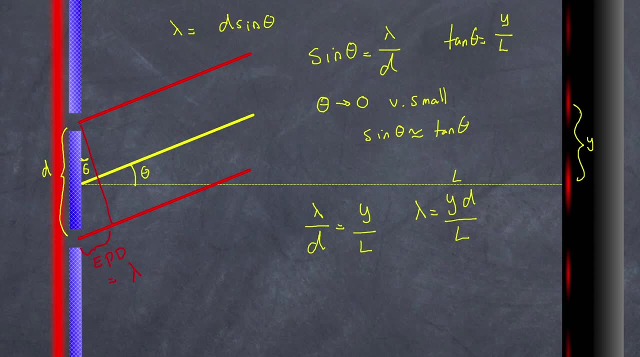 more multiple maximum, then you'll have one maximum here and so that again, to be a value of m of is equal to one, and over here, second matrix is gonna m equals the two. so what we can do also is put an m in front of it to suggest that the different maximum will have different values for angle. 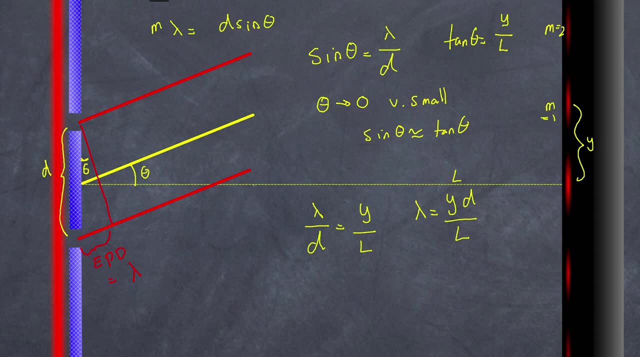 to keep you the same wavelength ever. j is. oh, thenéisousp Lemaitre's flux. does that corporation, that irstion that's going to equal the drama of the only difference to the distance. well, we've got an length Now. can we now use that information to determine the wavelength of light? And let's do. 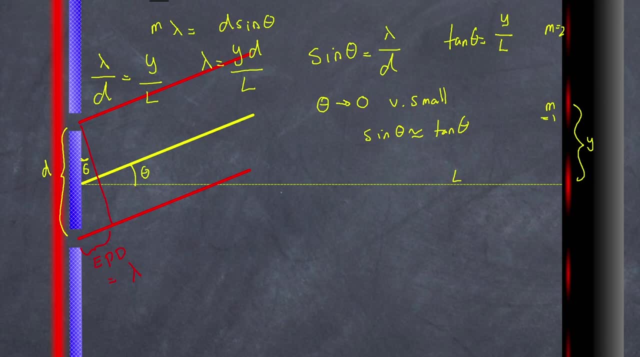 that. And now let's have a look at the mathematics Now. in the lab I worked at L to be equal to 4.332 meters, My distance was going to be equal to 300 micrometers And the other variable was: 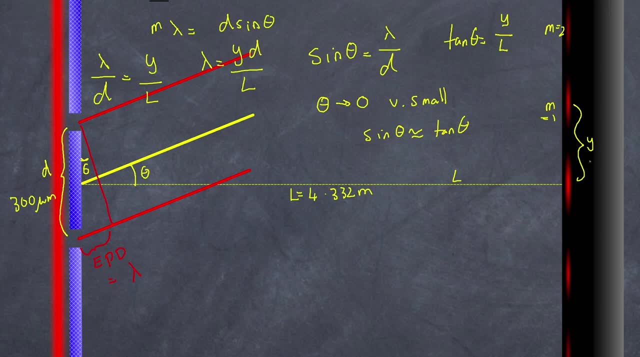 this distance here, which I stated was around 8 millimeters, Using that calculation that we have here, lambda is equal to 8 by 10 to the power of negative 3 multiplied by 300 micrometers. So that's 3 by 10 to the power of negative 7 meters over the distance 4.332.. And that gives me a value. 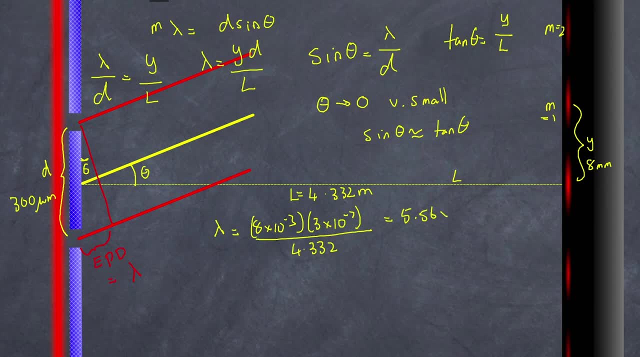 of 5.56 by 10 to the power of negative 7, or another way of describing this is: this is 556 nanometers. I know the value of the red laser and this standard laser has a wavelength of 632.8 nanometers, So you can see that my value is a. 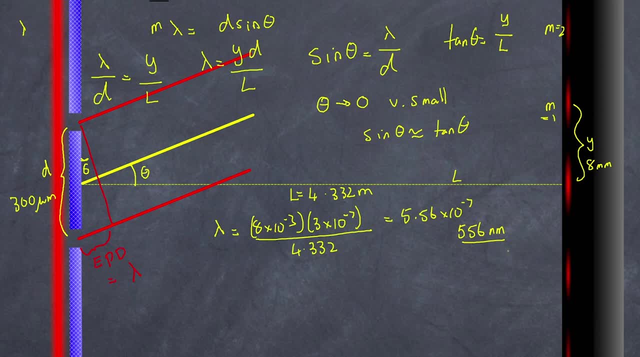 little bit out. In actual fact, I'm getting an approximate 12% error. Now, where is that error creeping in? Well, the biggest error is actually my determination of my separation between the maxima. So if I were to redo this calculation and say I was actually going to estimate it at 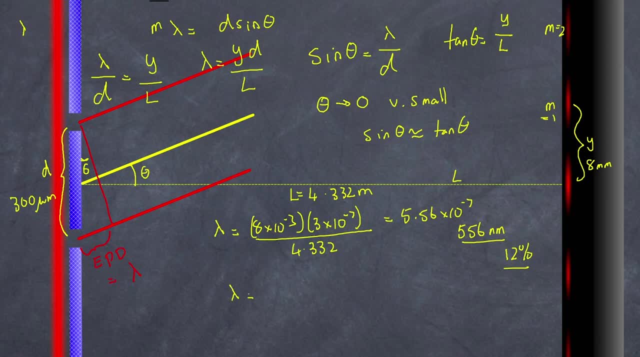 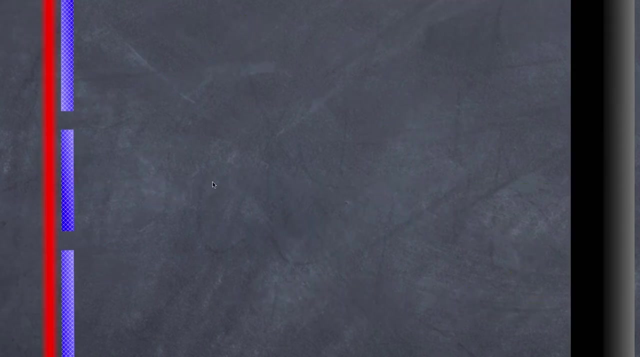 nine millimeters, my new wavelength now becomes 6.23 by 10 to the power of negative seven, that's 623 nanometers, And now I have a 1.5% error. So now one last little look at our double slits, And in this case I want to look at conceptually what 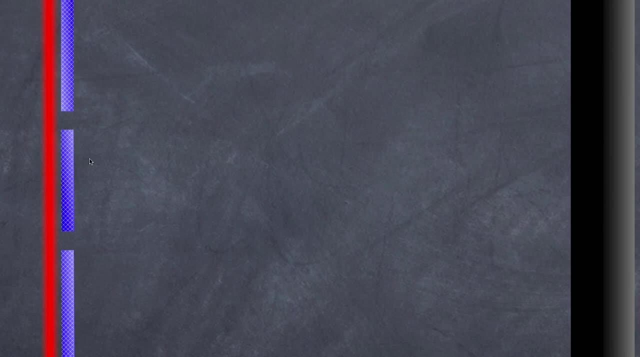 happens if we change the color of the light. So here I have my red wave. we established that produces, of course, our interference patterns like. so, But what if I instead have red? I have green light. If you remember, our relationship is that the wavelength is equal to d sine theta. 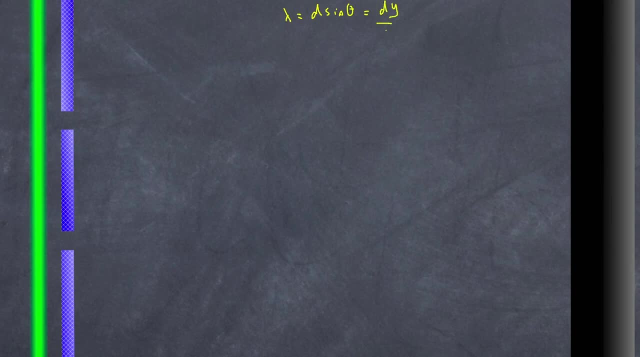 which is equal to d sine theta, which is equal to d sine theta, which is equal to d sine theta. So if I want to see the difference between the maximum and maximum, I have to get smaller as well. So if my wavelength gets smaller, then this gets smaller. Now my slit separation is still the same. 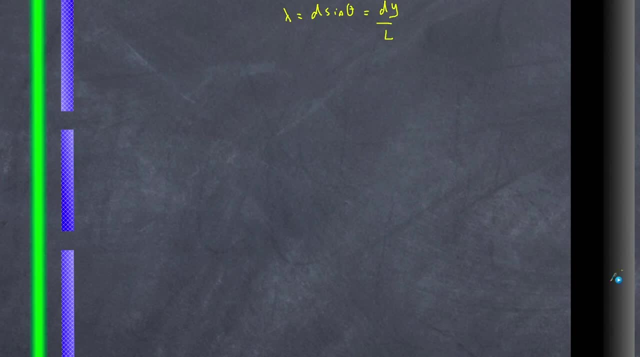 my length is still the same, So my separation between the maxima has to get smaller as well. So, in other words, my spots will look like this: Now, if I were to look at blue light, my spots would be closer again still. 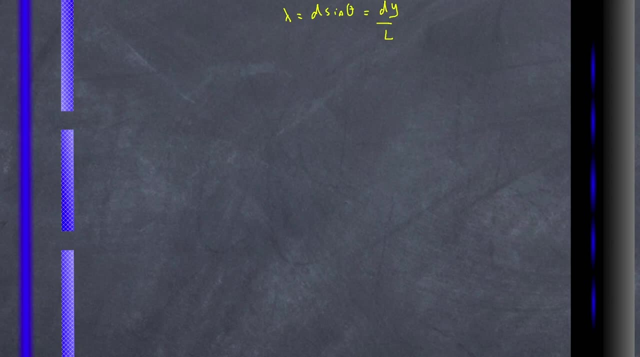 Now this is not particularly obvious, But what if I were to have all three lights at the same time? Well then, of course we'll get these sorts of spots like this, But you need to remember what we see is a combination of those colors. So this, in essence, is white light. And when? 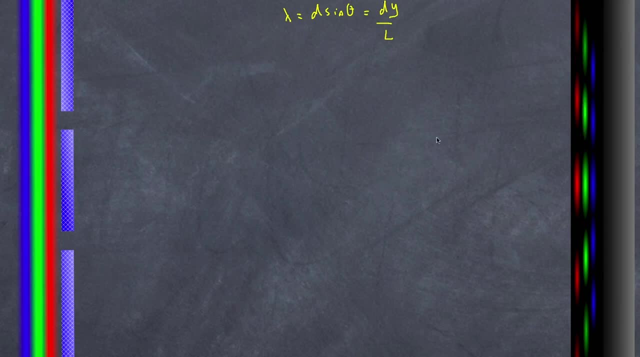 white light passes through, the different aspects of white light will produce interference patterns, patterns that are different. Now, if you look carefully in this section, here we're getting red but we're not getting any green and very little blue. Over here we're getting a sort of